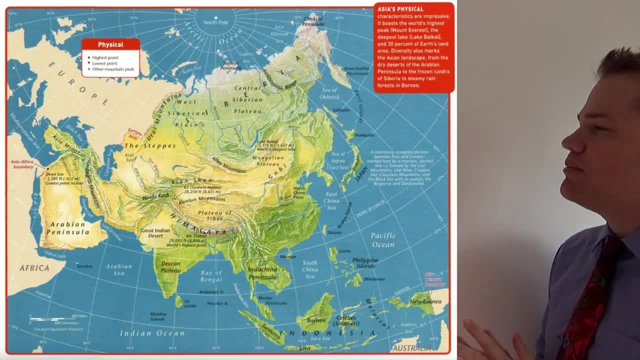 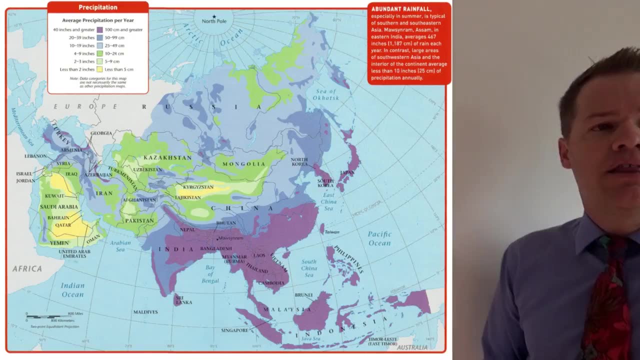 rivers, mountains. that's called a physical map. and the last category category of maps is the thematic map. a thematic map shows us distribution patterns, things like climate, population density and so on. I'm not going to go into too much detail about the map, but I'm going to show you a map of the 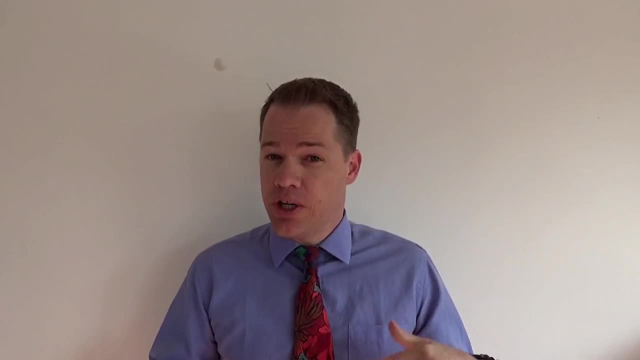 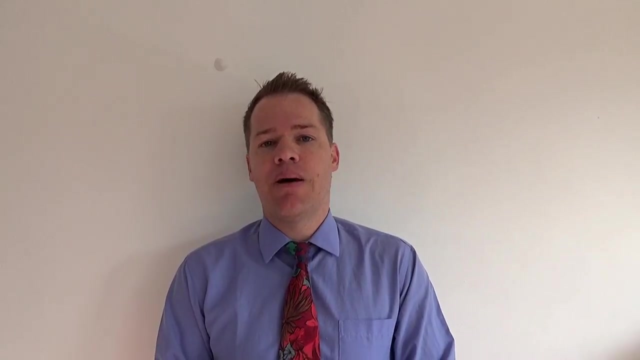 first time you want to know which area is represented by the map. the next thing we need to know is: where is north on the map? now, for every standard map that exists, north will be at the top of the map. as you can see, this is standard map. 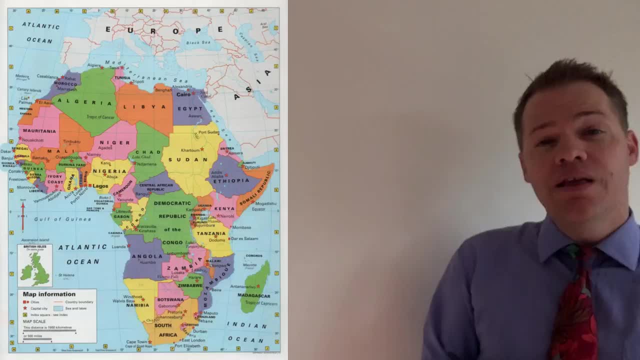 north is at the top, south is at the bottom. there are, however, exceptions and when we look at the map, we see that north is at the top, south is at the bottom and where North is not at the top, there will be a sign like the one you see on. 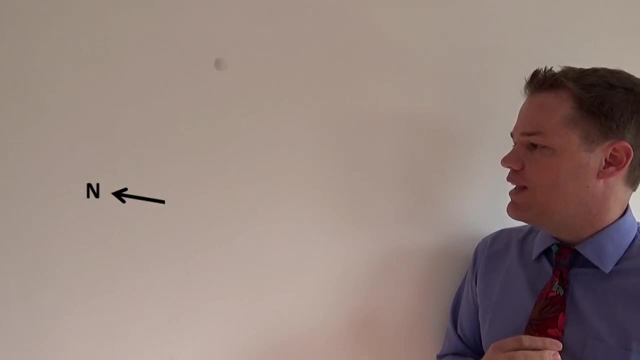 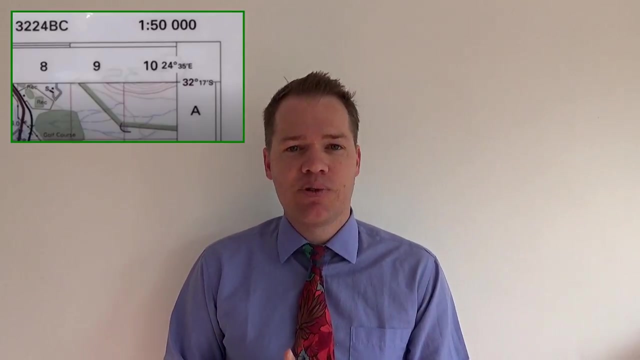 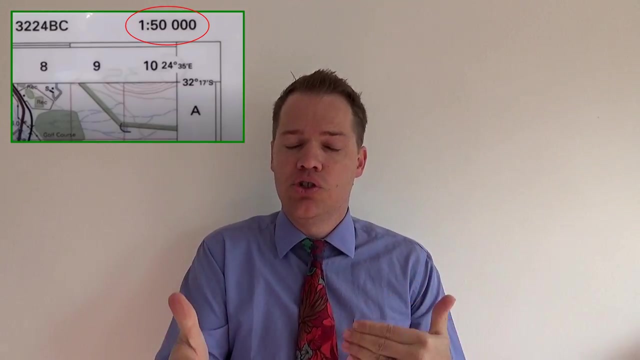 your screen indicating where north is. so now that we know where north is, it's important to identify the map scale. what is a map scale? a map scale is something that tells you how many times a piece of land was shrunk so that it can be used as. 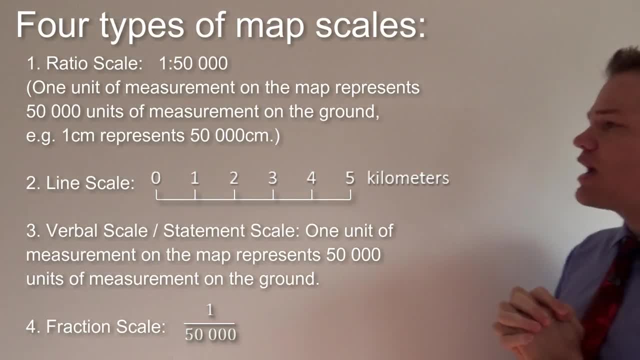 a map. on your screen you'll see examples of map scales. one at the top is the ratio scale, the one that's at the top is the ratio scale and one at the bottom is the measurement scale. below it is a line scale and the one below the line scale is a verbal scale and the one right 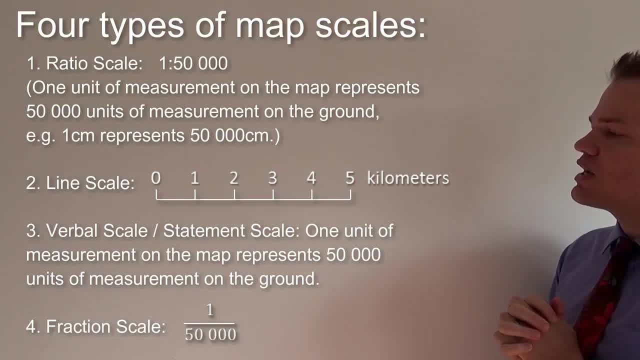 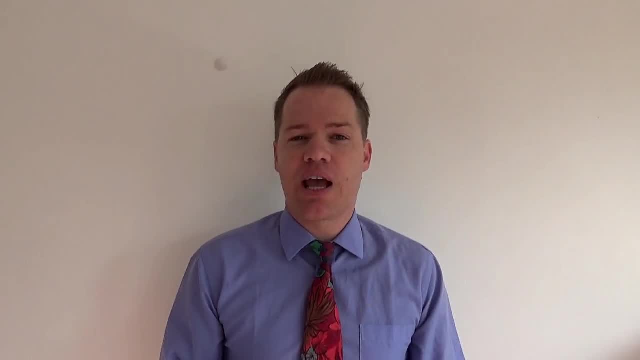 at the bottom. it's very similar to the ratio scale is a fraction scale so, like I said, I'm not going into any detail. I've posted videos on different types of scales, so feel free to click the links in the description below to see those videos. next thing we need to know is- and this is: 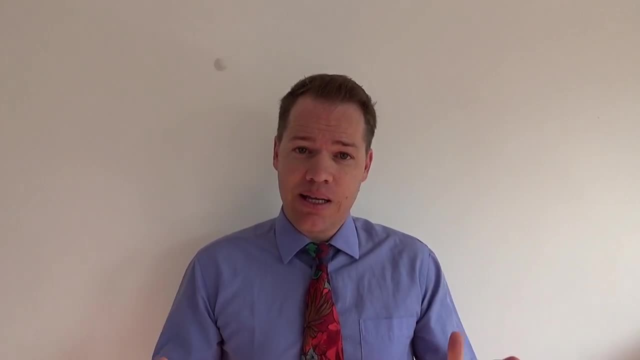 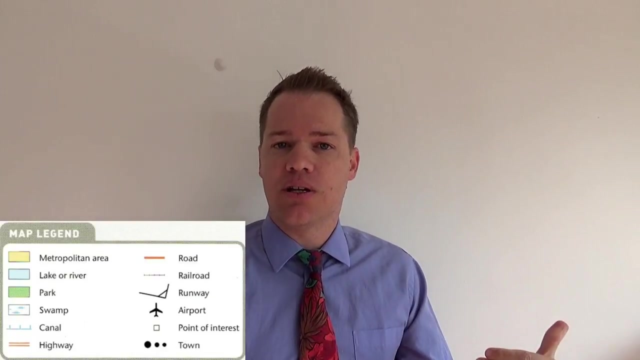 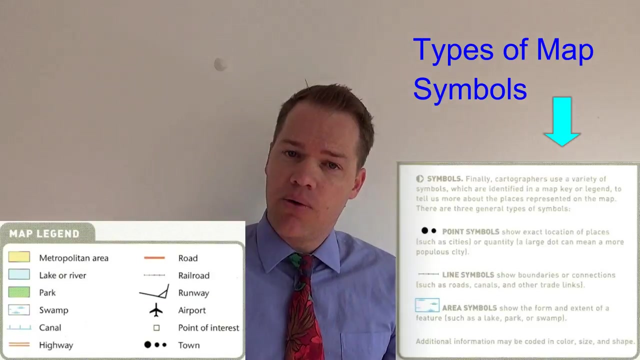 very important. this part of the video is about actual map reading. now, the map key or the map legend is like your dictionary, because on your map you'll see symbols and lines, as I've said before, and you might not know what these represent. so if you look at the key or the legend, you will see. 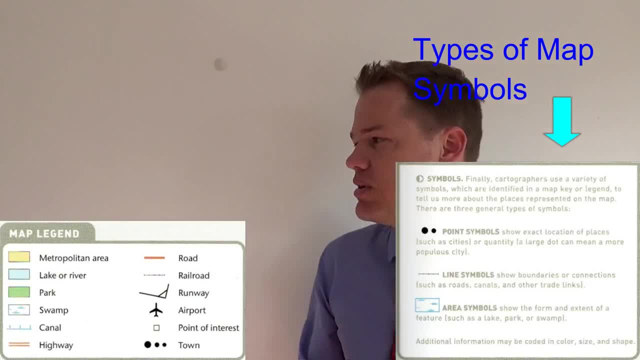 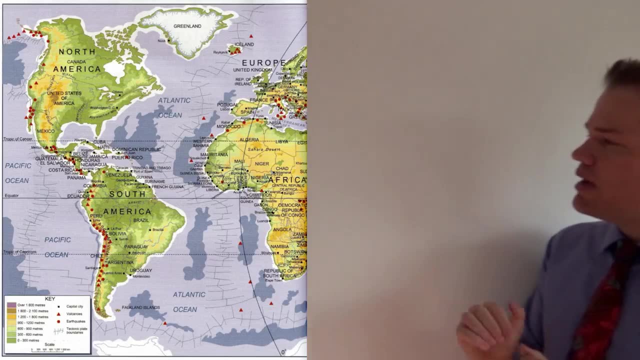 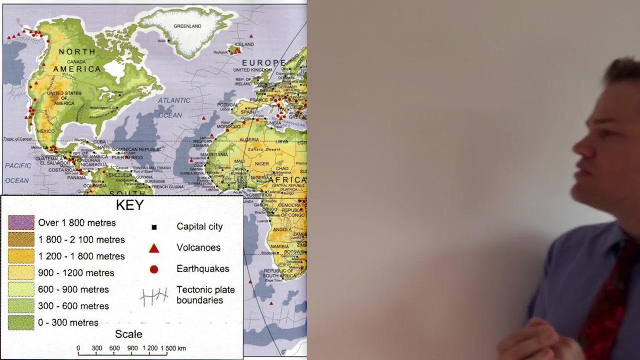 exactly what these lines and symbols mean. so on the screen there's a map and we have lines and colors and symbols. so let's zoom in on the map key, or the legend, and there they give you the meaning of each of these lines, colors, symbols and shapes. so one of the the first things I noticed when I look at the map- 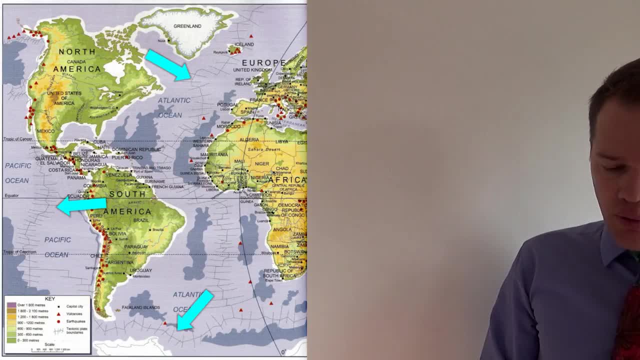 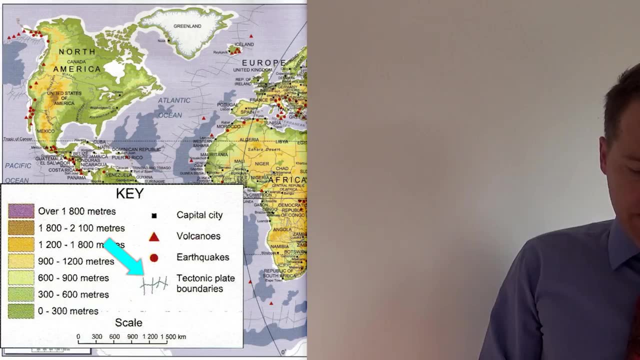 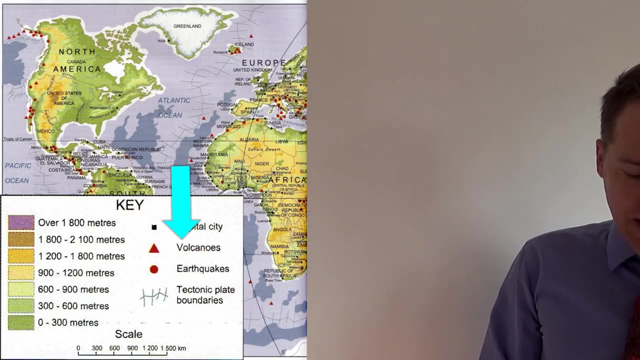 are these lines, and so what do they mean? if we go to the key, we'll see it's where tectonic plate boundaries are. then I see these red triangles. what do these red triangles mean in the key, it tells you exactly what they mean. they are volcanoes. and so we can carry on. 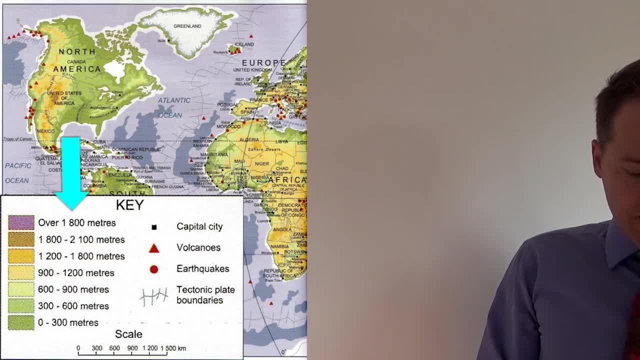 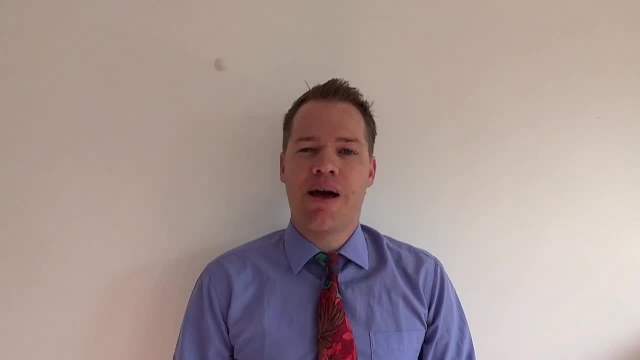 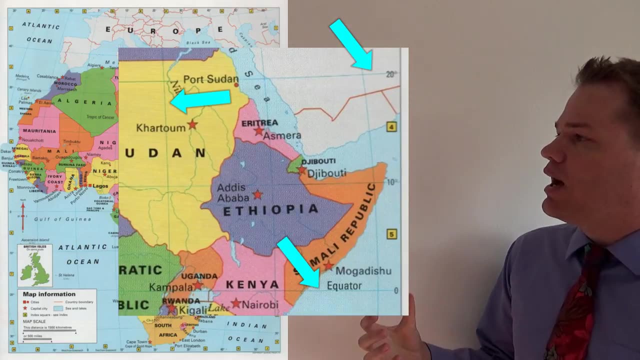 you also see the different colors, and so the different colors tell you the height of the land. the next thing you will notice on a map are these grid lines. now, these grid lines are there to just help us identify exactly where certain places are located. so if we say a certain place, 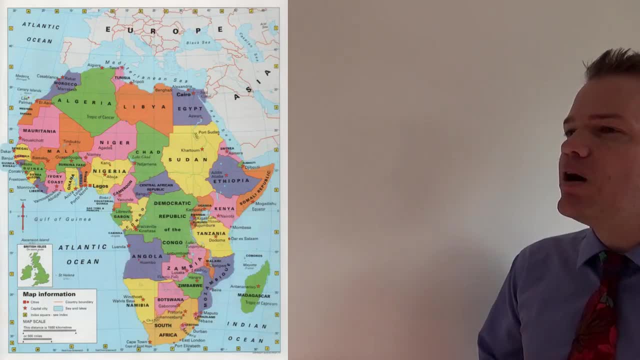 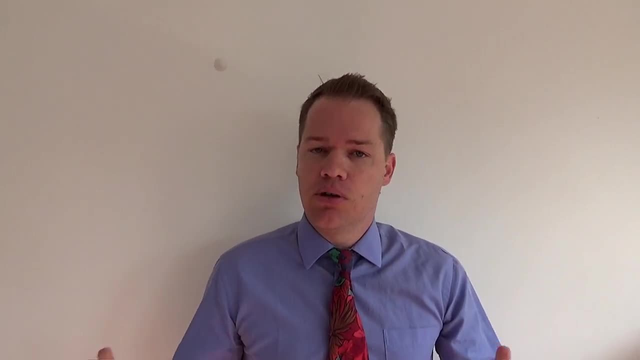 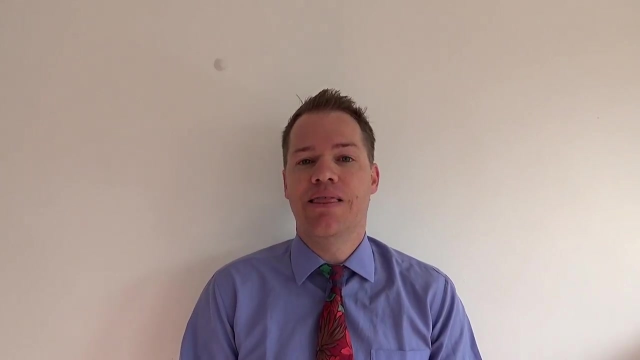 is exactly on the equator, then we know more or less where to go and look for that place. i've also posted videos on coordinates, lines of latitude and longitude, where i explain how to plot places and find the location of certain places by looking at these lines of latitude. 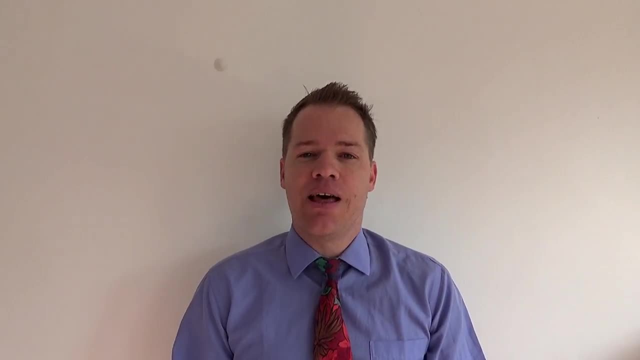 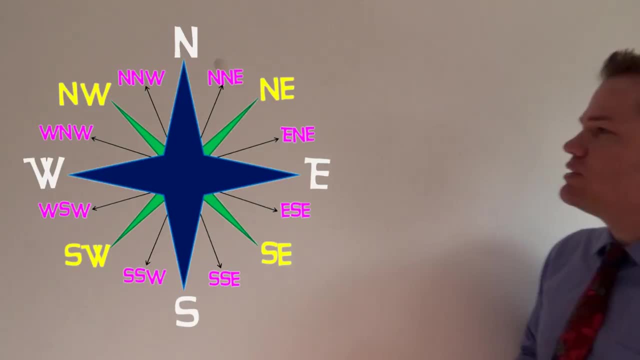 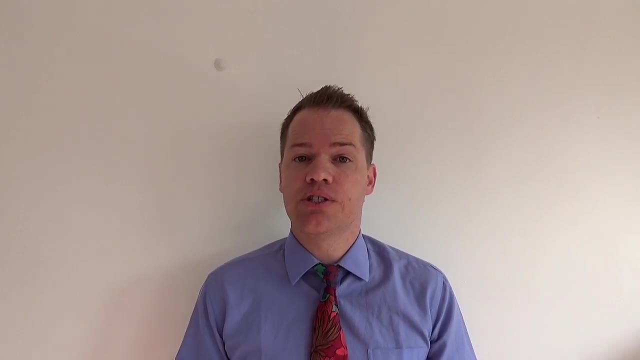 or less like this, and important especially when you travel, you want to know in which direction you are traveling. thanks for watching. if you have any questions, feel free to ask your question in the comment section below. also go and look at the the description of this video, because there you'll find many links to a. 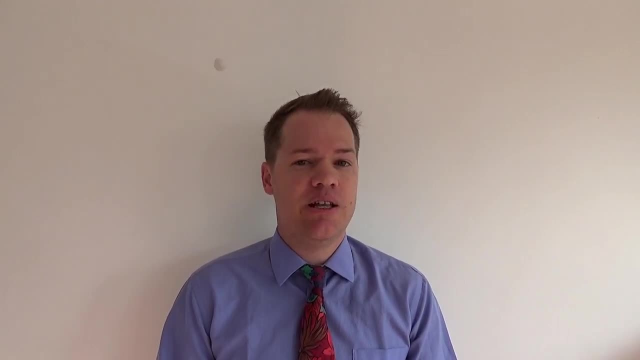 variety of geography map work videos. that would really be helpful, so feel free to subscribe. see you next time. goodbye.